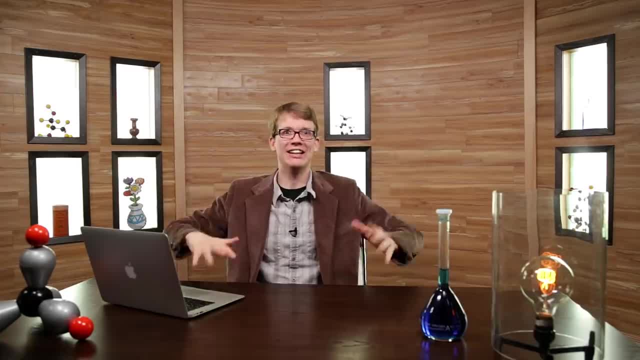 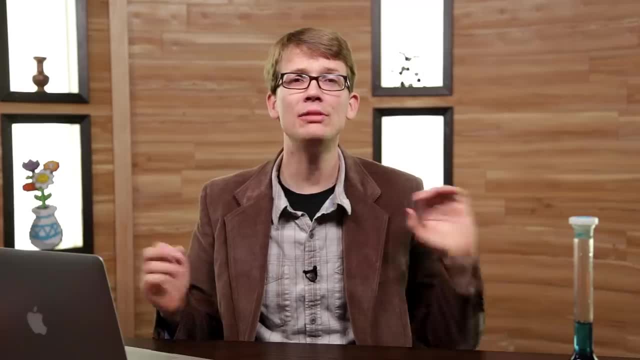 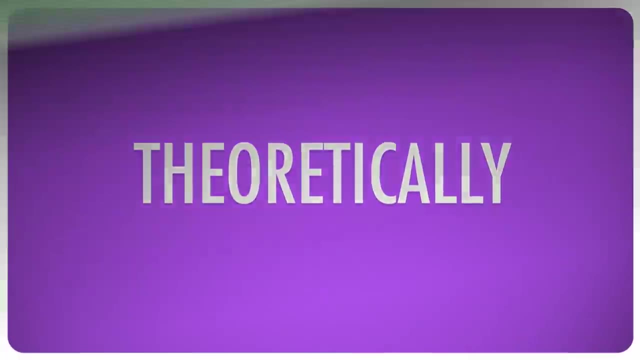 You can't look cool while you're feeling it, but you can feel it. It's there, those little molecules and atoms bumping around against your hands as you wave them around. Feel it. Are you doing this? I've got good news and bad news about gases. First, the good news: when they're behaving themselves, it is extremely easy to describe their behavior theoretically, experimentally and mathematically. 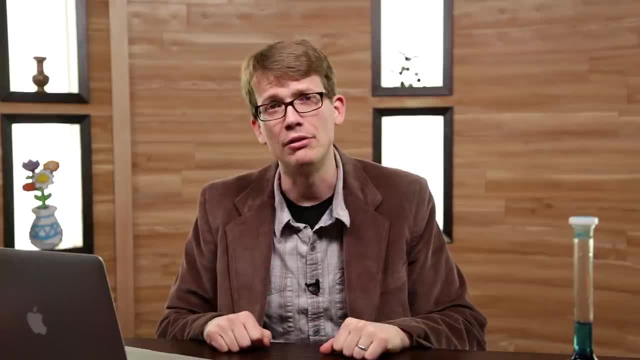 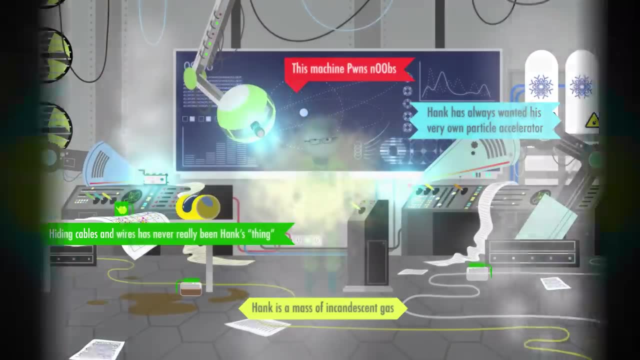 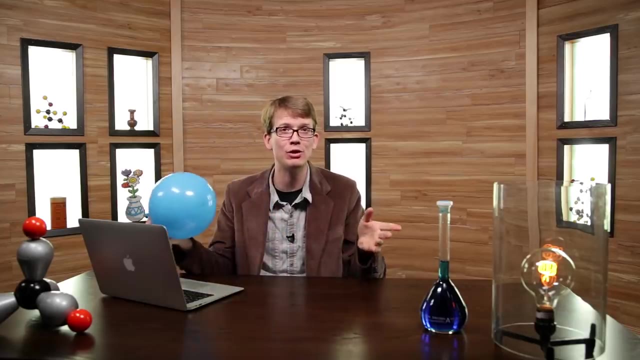 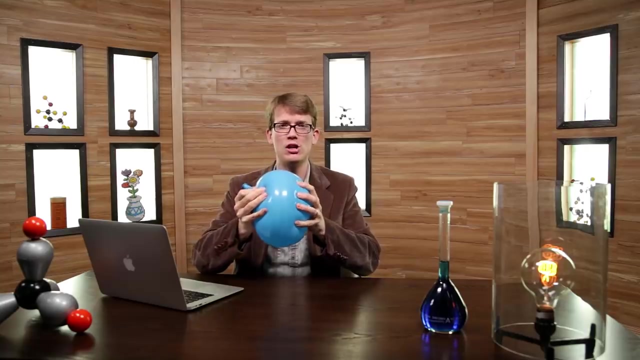 The bad news is they almost never behave themselves. The first mathematical description of the behavior of a gas was the link between pressure and volume. In a close-up I'll show you how to describe it. In a closed system like the inside of this balloon, when we decrease the volume of the balloon, the pressure inside goes up. 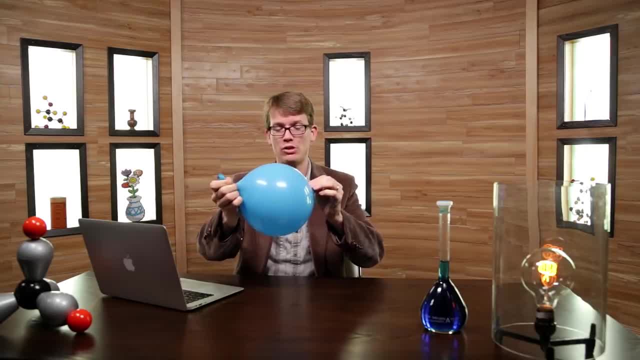 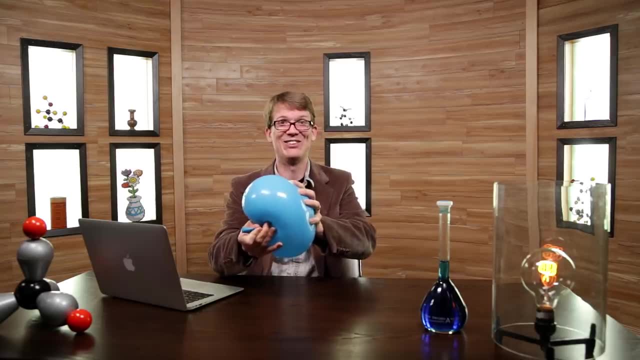 And if we could somehow expand the balloon, then the pressure inside the balloon would go down. If I keep pushing on it, the pressure inside might go so high that it'll break. I hope I can't do it. It's a very strong balloon. 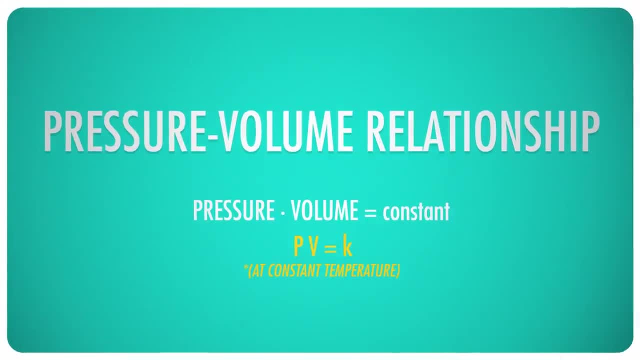 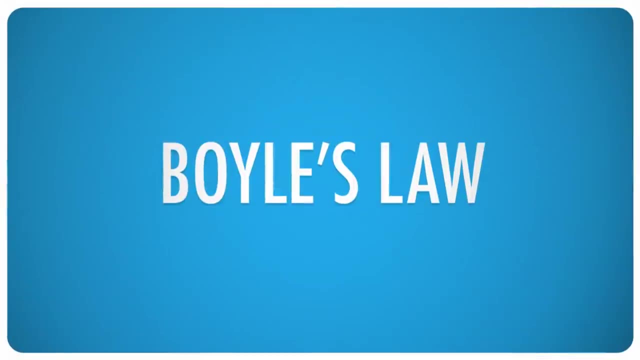 The relationship here is a simple one. When you multiply the pressure and the volume together, you get a constant. As long as the temperature and the amount of gas stays the same, so does that constant. It's called Boyle's Law, and it was a pretty big deal back in the 1600s. 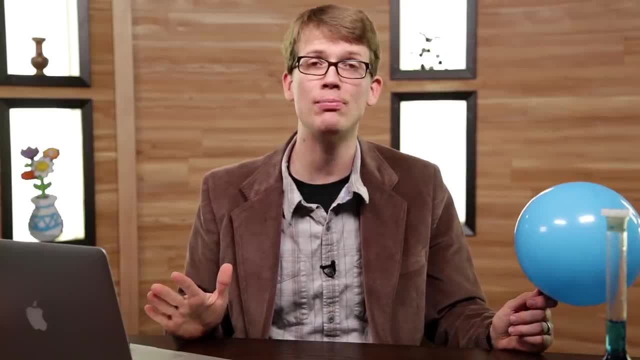 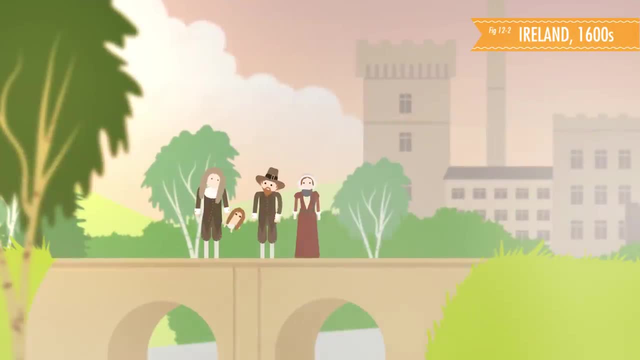 It's also one of the greatest scientific misattributions of all time. Robert Boyle was a super-rich Englishman raised in Ireland. His father was so rich that he paid another family to raise his children, I guess because he was too busy administering lands, or something. 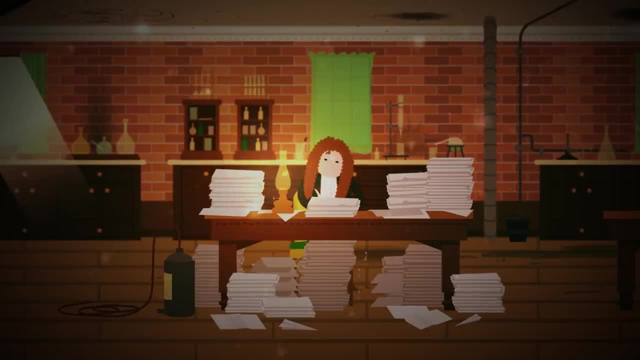 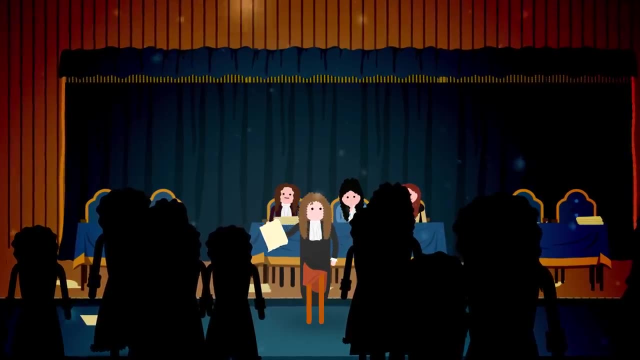 Boyle had lots of great ideas about science and chemistry, His most important one- and this is arguably even more important than Boyle's Law- being that chemists should publish papers not on what they feel is correct, but rather on theories that have been backed up by experimentation. 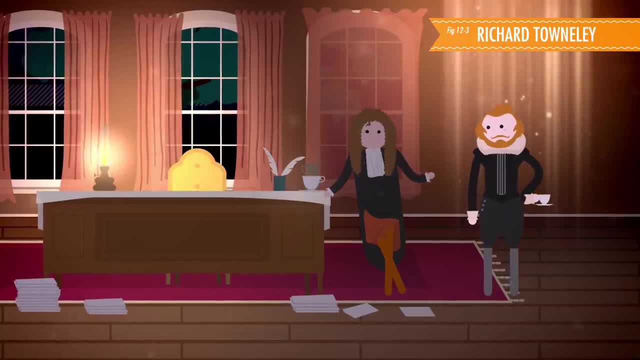 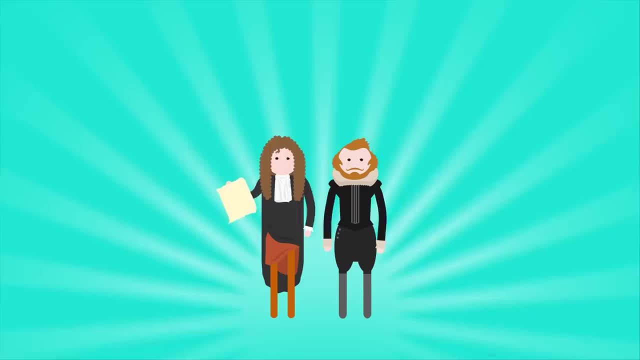 Richard Townley, a wealthy but considerably less wealthy Englishman, struck up a relationship with Boyle, telling him about some of his work that would disprove one of those but-it-feels-right kind of chemists. Boyle published a paper mentioning that work, which he called Townley's Hypothesis. 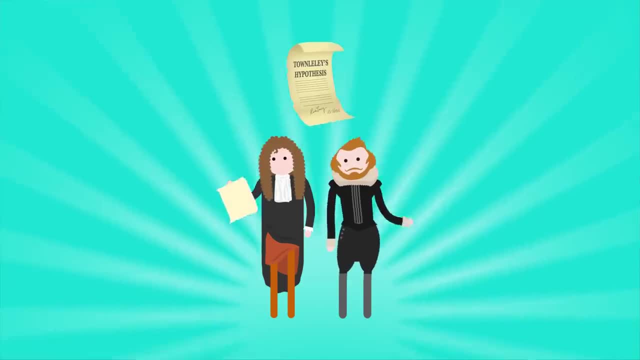 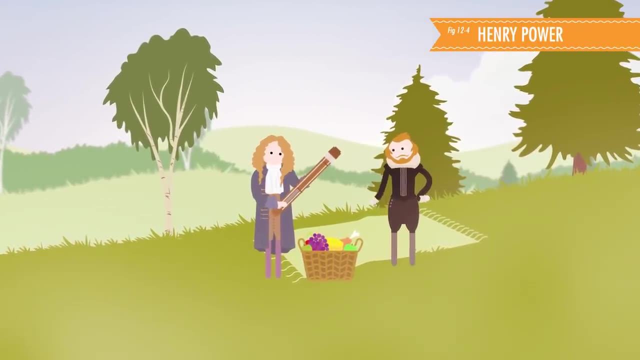 but which ended up, because of Boyle's superior scientific standing and possibly his wealth, being called Boyle's Law. But here's the really messed up thing: The experiments that led to the creation of this theory were actually done largely by Townley's family, friend and physician. 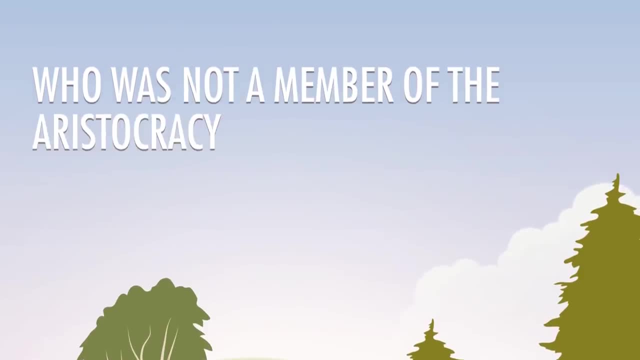 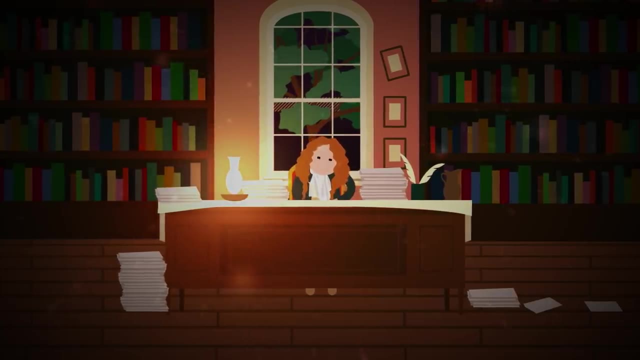 Henry Power, who was not a member of the aristocracy at all. He was just a working class scientist. Power was working on a publication that would have snared him the position as discoverer of the relationship between the pressure and volume of a gas. 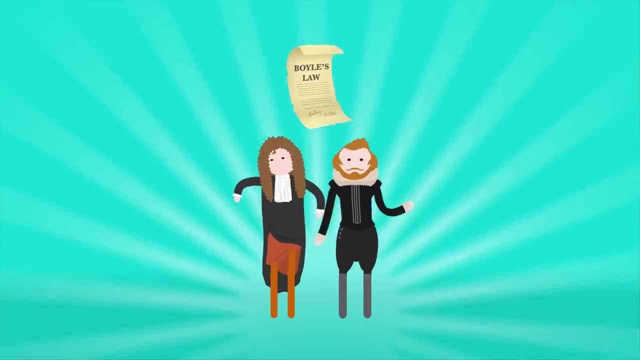 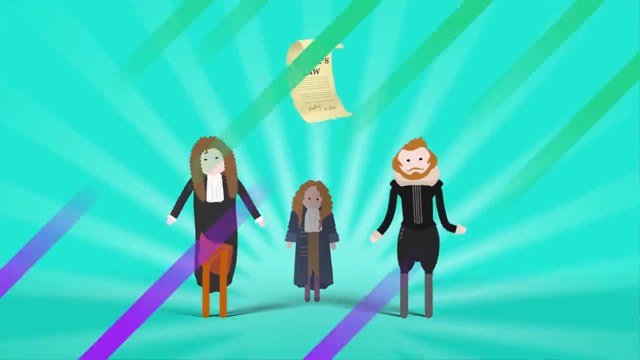 But Boyle, having discussed the ideas with Townley, privately published his first attributing Townley as the sole researcher, ensuring that Power's contributions were all but lost to history. Henry Power's Wikipedia page didn't even mention Boyle's Law until a few weeks ago. 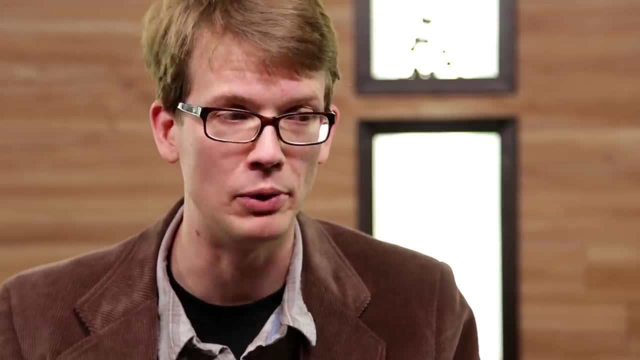 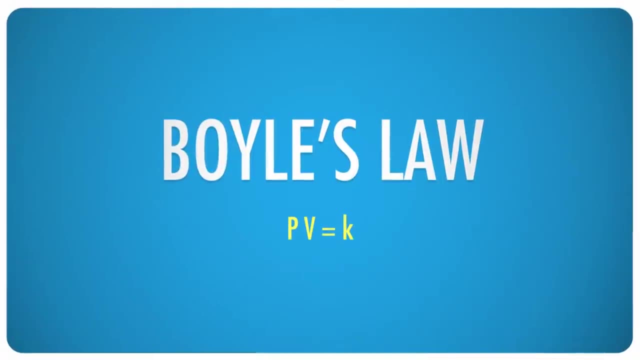 when I personally added a paragraph about it, with proper citations, of course, But no matter who thought it up or who had got named after Boyle's Law, it's pretty cool. For a given amount of gas at a constant temperature, pressure, times, volume always equals the same number. 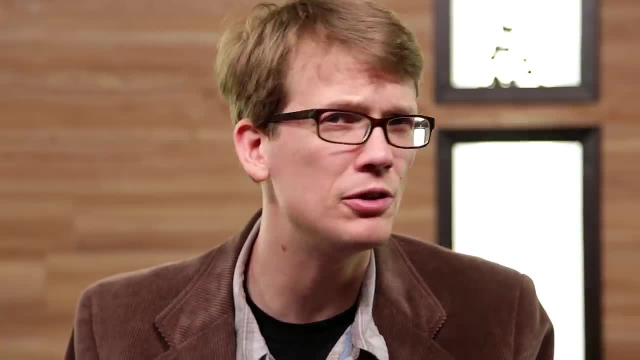 But where is that constant coming from, And why is it different for different amounts of gas at different temperatures? Well, it was more than a hundred years before we'd figure out the answers to those questions. Well, it was more than a hundred years before we'd figure out the answers to those questions. 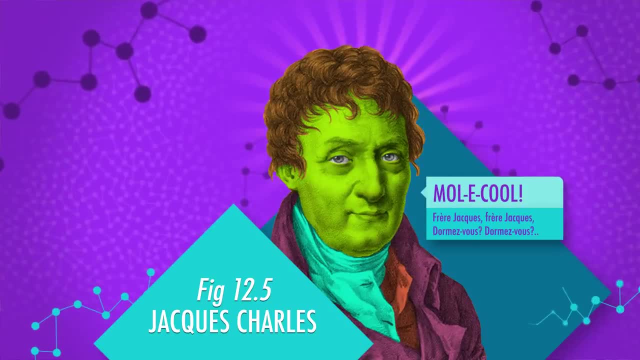 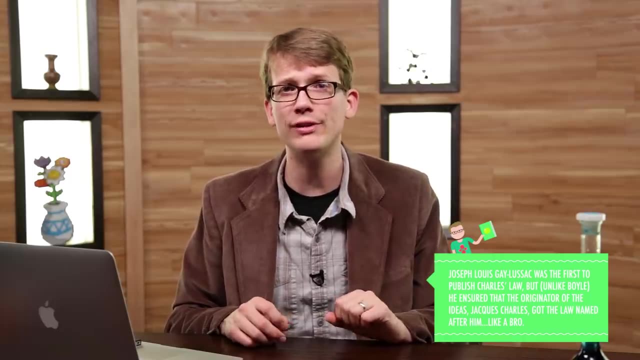 with the help of a Frenchman, Jacques Charle, and our old Italian house-elf friend, Amadeo Avogadro. Charle and Avogadro created equations much like Boyle's Law, with two features of a gas being linked directly together by constants. 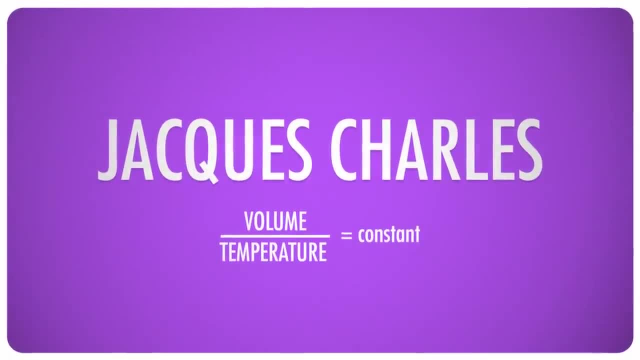 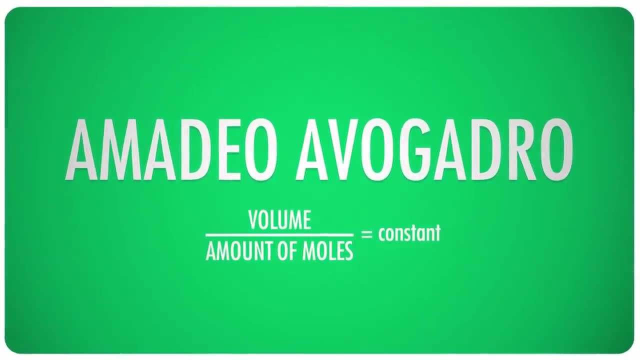 Charle discovered that volume divided by temperature equals a constant as long as the pressure remains the same. and then Avogadro figured out that volume divided by the number of moles in the container at a constant pressure and temperature gave yet another constant. 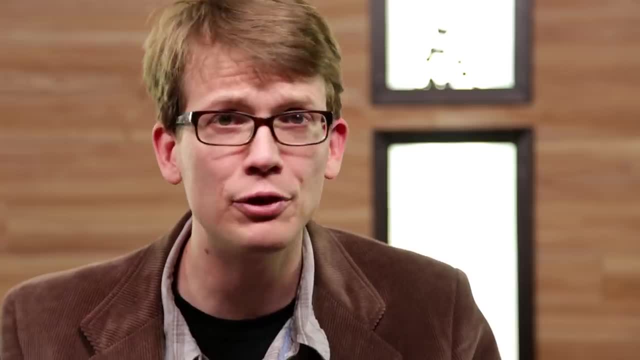 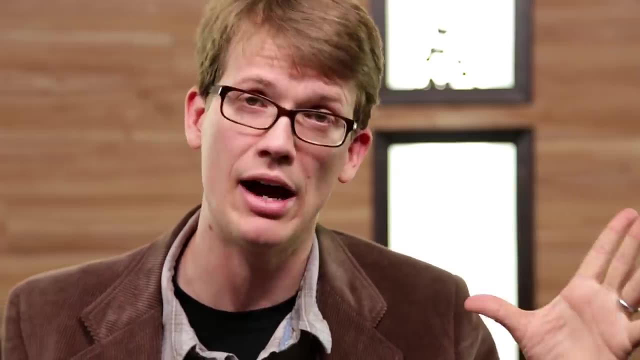 But here's the crazy cool thing: all of these scientists were basically dealing with a different form of the same equation, An equation that we must never forget and is going to be stuck in my head until I die. And here's how it works. 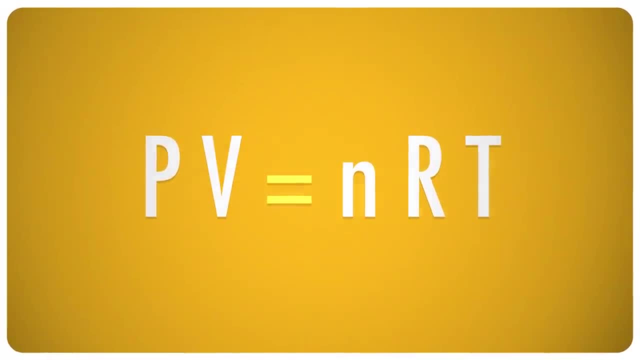 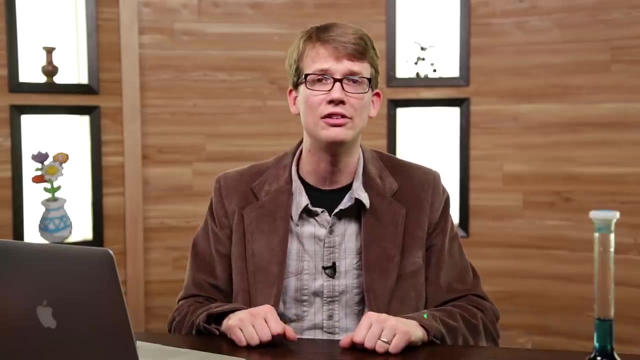 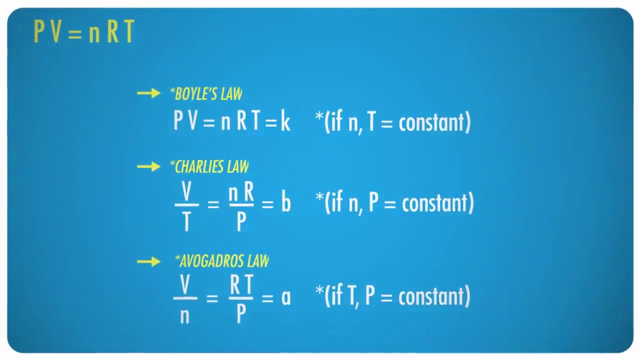 Pressure times. volume is equal to the number of moles of substance times a constant times temperature. PV equals nRT, the ideal gas law which works for all gases as long as they behave themselves. Now here's the cool part: using this equation, we can show how all of these chemists were dealing with the same relationship. 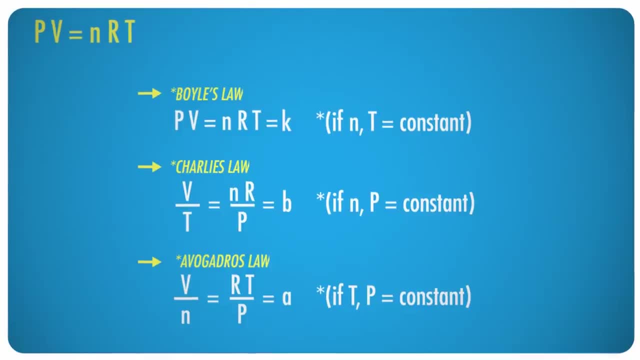 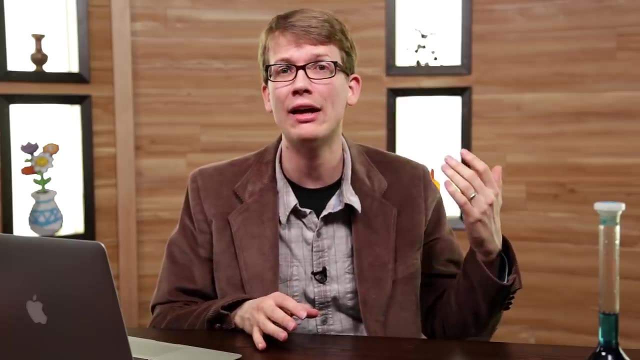 They were just clumping various variables together in different orders. All of the chemists we just mentioned, Charle Avogadro and Boyle, or more properly, Townley and Power, figured out their contribution to the ideal gas law experimentally. 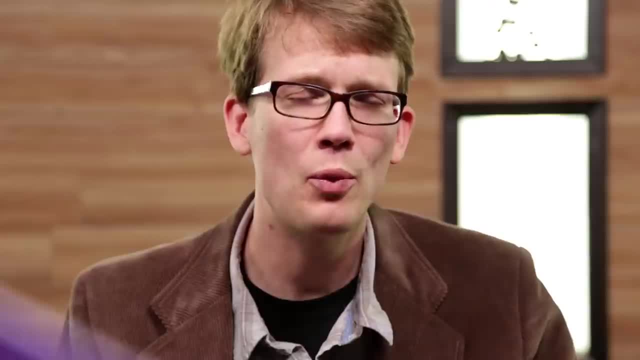 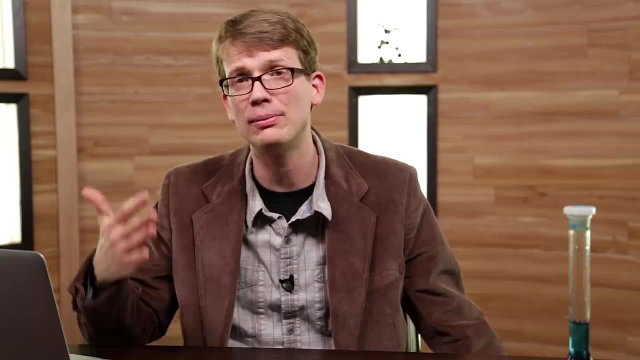 But more interesting to me is that it can be understood theoretically. First we have to understand what each of these variables actually mean. In that same way, the atoms and molecules that make up gases are bouncing against things applying pressure to them. This balloon is inflated because the molecules are bouncing around inside of it, bumping into the inside of the balloon. 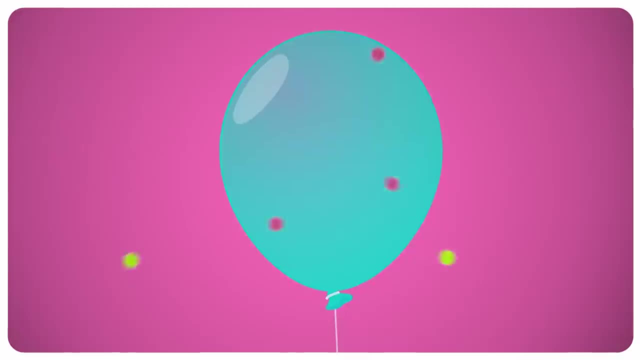 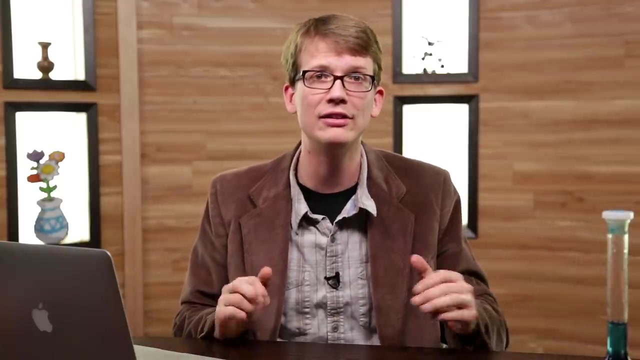 harder than the molecules bouncing off the outside of the balloon. Scientists generally measure pressure with the SI units of force, newtons per area, meters squared, which is shortened to pascals, But since pascals are so tiny, we either use kilopascals or we use the pressure here on Earth at sea level that we call one atmosphere or one atm. 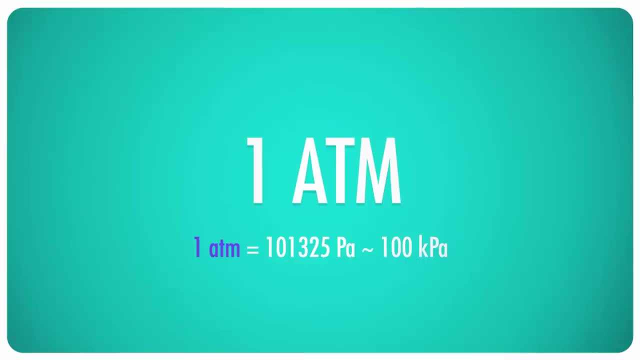 Completely by chance. one atmosphere is equal to 101,325 pascals, but that's so close that we often just say that one atmosphere is 100,000 pascals Or 100 kilopascals. Volume is the amount of space particles have to exist inside of. 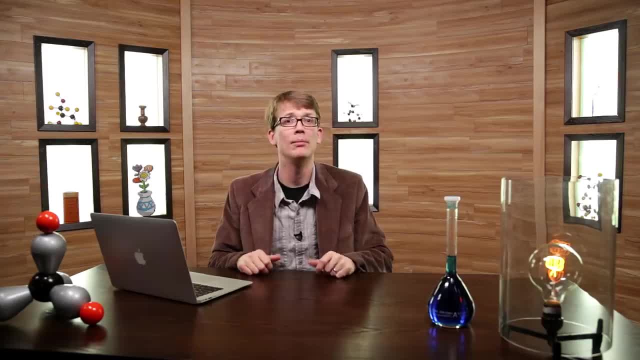 So, yeah, that makes sense. When the volume goes down, the pressure goes up Because there are more particles in a smaller space and they'll each hit the walls more often. N is simply the amount of gas, the number of moles in the system. 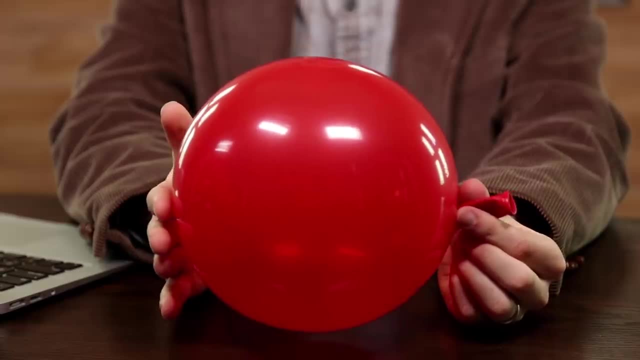 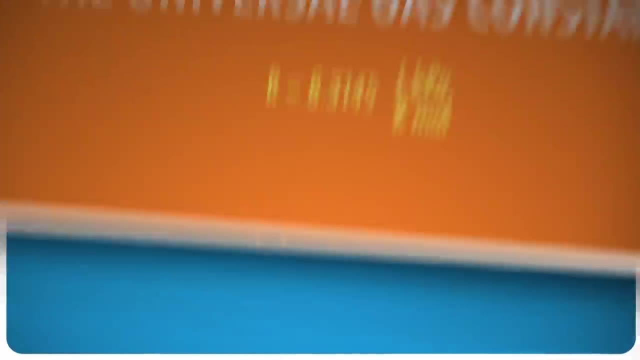 Here I am decreasing the amount of gas in the system and in response the volume is decreasing, obviously, But so is the pressure inside the balloon. R in the ideal gas law is called the universal gas constant, even though, as we will see in a coming episode, 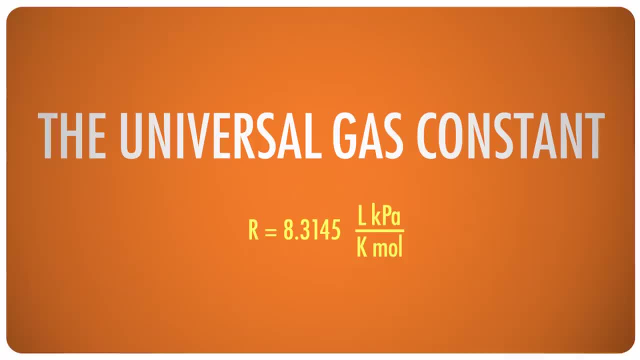 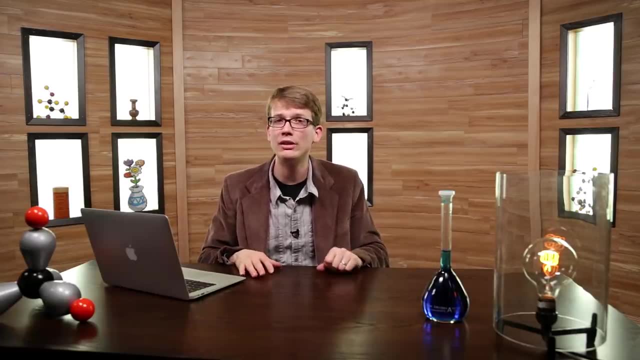 it is neither universal nor constant. It's 8.3145 liter kilopascal per kelvin. mole Temperature is experienced by you and me as hot or cold, but at the atomic level it's kinetic energy, literally how fast or slow the average particle is moving. 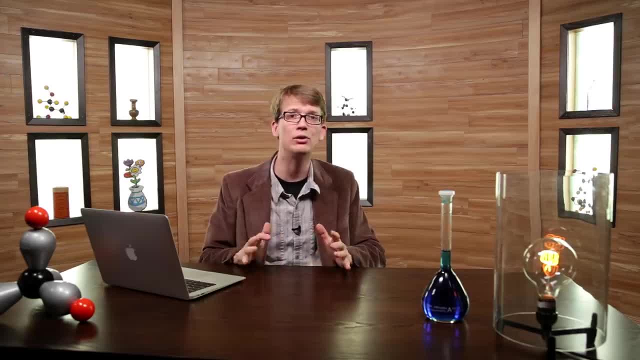 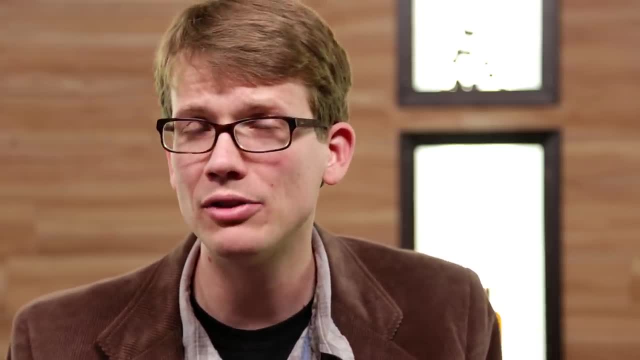 So if temperature goes up, so will the pressure, as the particles are moving faster and thus will run into the sides of the container more often. So now we know about all of the little bits of the ideal gas law, so let's take a look at it in action. 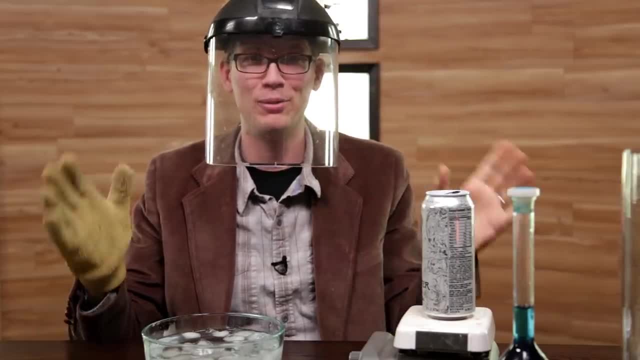 We here at Crash Course generally like to be very safe. This is a little bit overkill here. I put a little bit of water into this soda can and now I'm boiling it. So instead of atmospheric gas in this can right now. 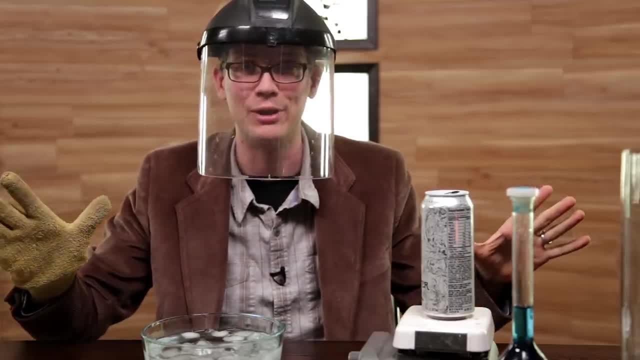 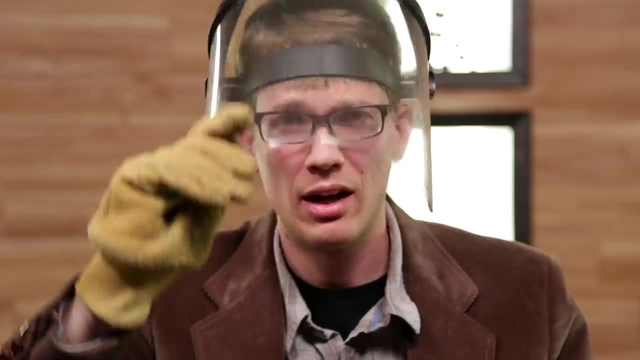 there's water vapor and it's hot and all the molecules are zipping around like crazy. We pick it up and we plop it down inside. Stop that, Oh, And it crushes itself. So what just happened there? 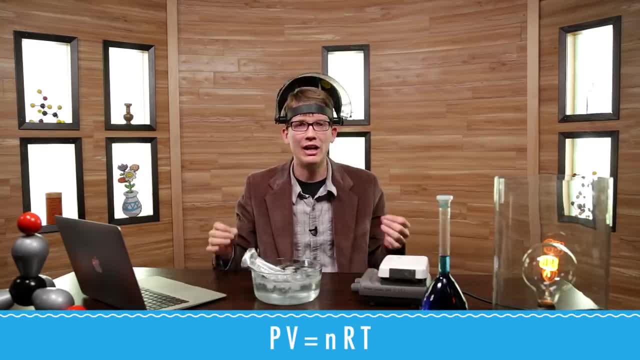 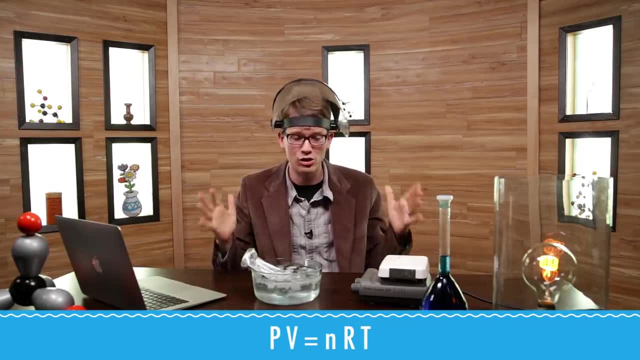 Well, let's see what the gas law can tell us. So which of these things are changing? Starting on the right hand side: R is constant, so that can't change. Constant gas- though that definitely changed- It drops like mad when it's exposed to the ice water. 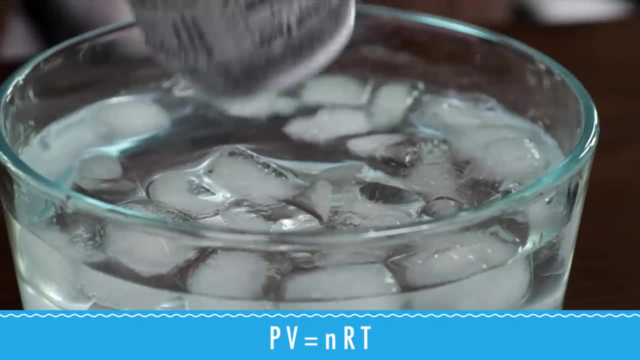 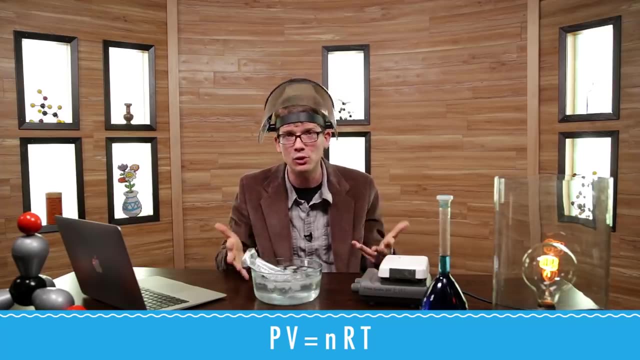 N is decreasing too, as water vapor is condensing into liquid water. It thus disappears from the gas phase. So the net result on the right hand side is a decrease, and that means the left hand side has to have a net decrease too. So on to the left hand side. the pressure does indeed drop because the lower temperature makes the molecules move more slowly, thus bumping into the sides of the can a lot less than before, And volume drops too, but not quite for the reason you might think. It's really that the pressure inside the can goes so low that the pressure outside the can, the atmospheric pressure, literally crushes the can. Now I understand that you probably don't think this is as cool as I do, but understanding the physical reality of atoms and molecules smacking into things, 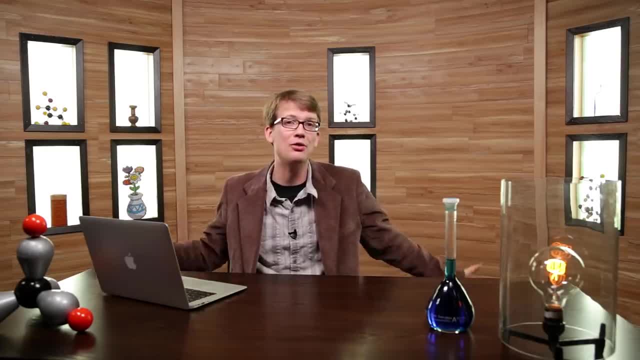 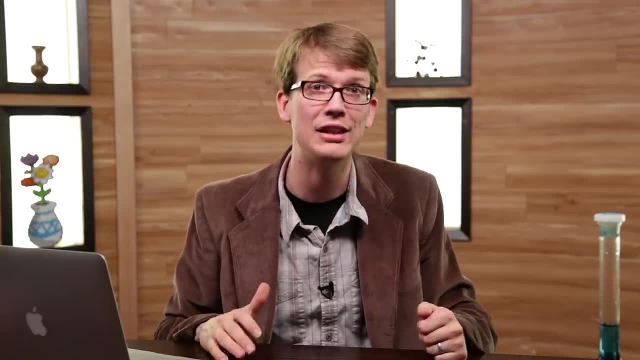 is a special kind of beautiful. for me, It's also pretty cool that if you know any three things about a gas, you can figure out the fourth using the ideal gas law. Of course, not all gases behave ideally and all gases deviate from the law at low temperatures or high pressures. 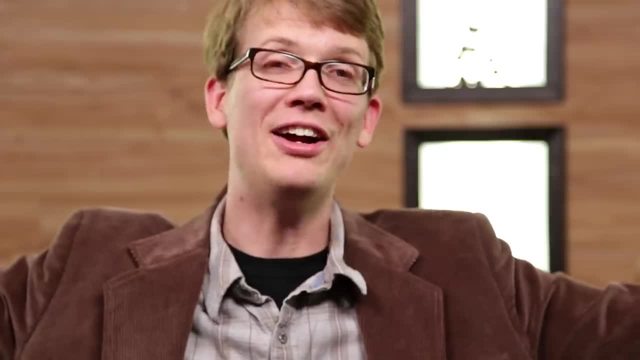 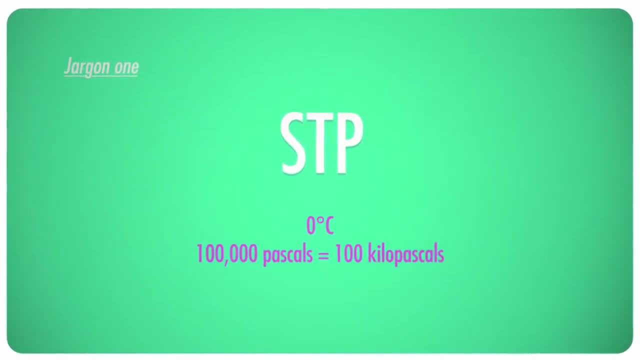 but we'll save that discussion for later episodes. Jargon fun time. STP means standard temperature and pressure, which according to the lords of chemistry is 0 degrees Celsius and 100,000 pascals or 100 kilopascals. 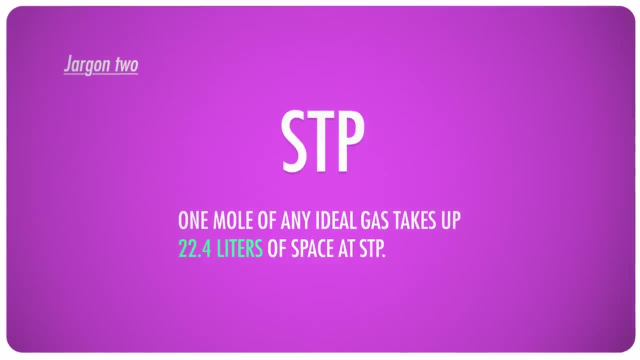 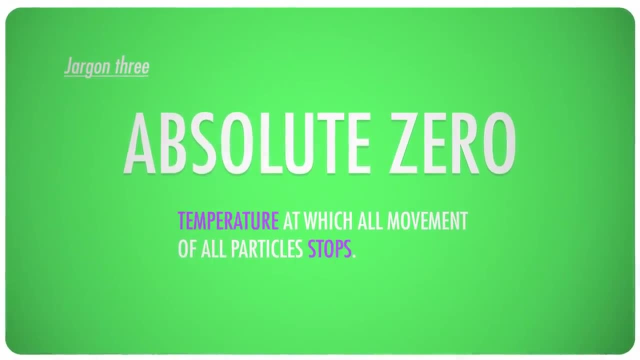 One mole of any ideal gas takes up 22.4 liters of space at STP, which is a fact that can simplify a lot of calculations. Absolute zero is the temperature at which all movement of all particles stops. It is 0 kelvins or negative 273.15 degrees Celsius. 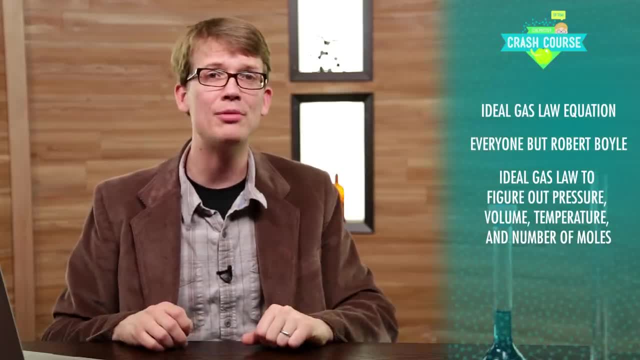 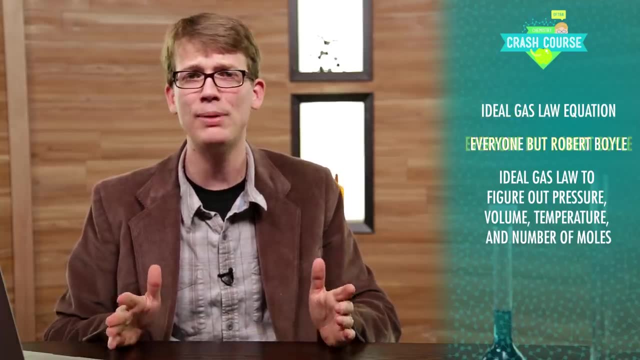 And that's all for this episode. Thank you for watching Crash Course Chemistry. I hope you were paying attention. You learned about how the work of some amazing thinkers combined to produce the ideal gas law, how none of those people were Robert Boyle and how the ideal gas equation allows you to find out. 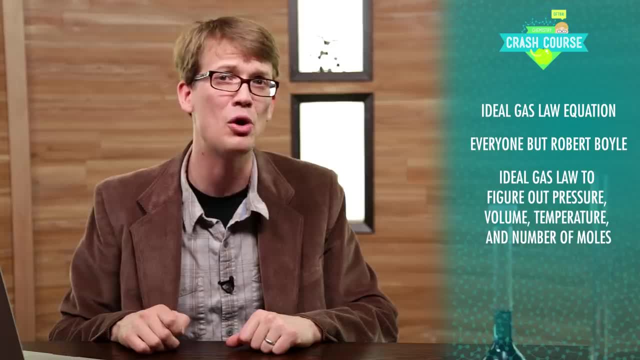 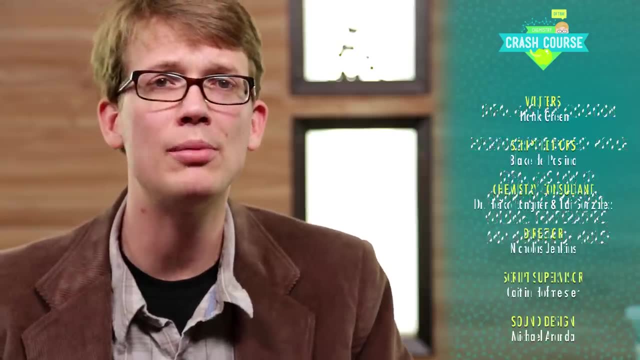 pressure, volume, temperature or number of moles. as long as you know three of those four things And you learned a few jargony phrases to help you sound like you know what you're talking about, This episode of Crash Course Chemistry was written by me. 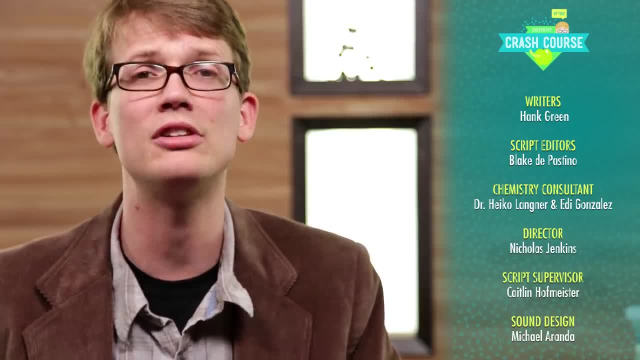 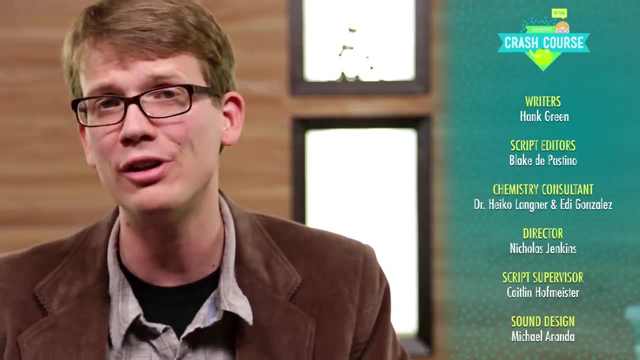 the script was edited by Blake DePastino and our chemistry consultants were Dr Heiko Langner and Edie Gonzalez. It was filmed, edited and directed by Nicholas Jenkins, Our script supervisor was Caitlin Hoffmeister and our sound designer is Michael Aranda. Our graphics team is Thought Cafe.